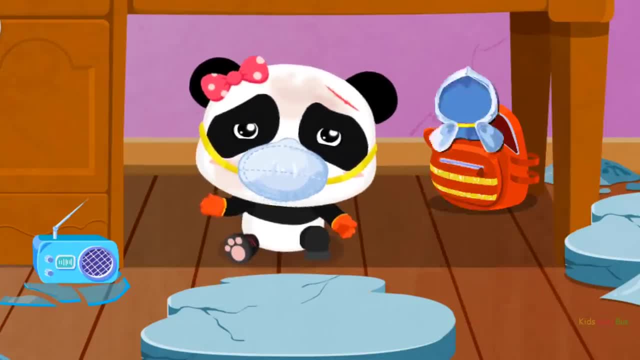 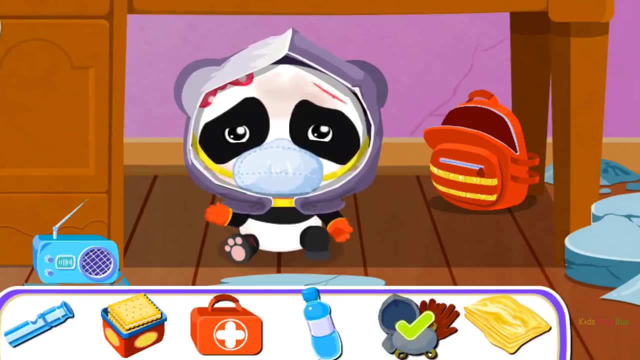 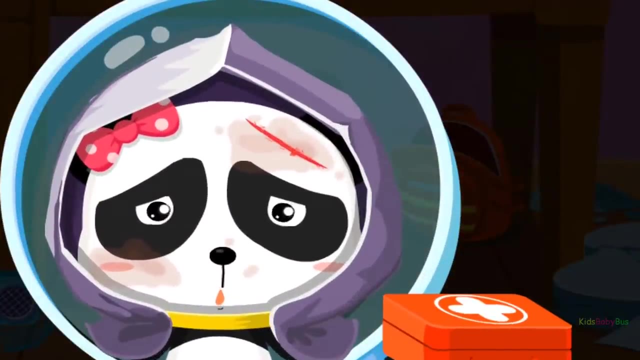 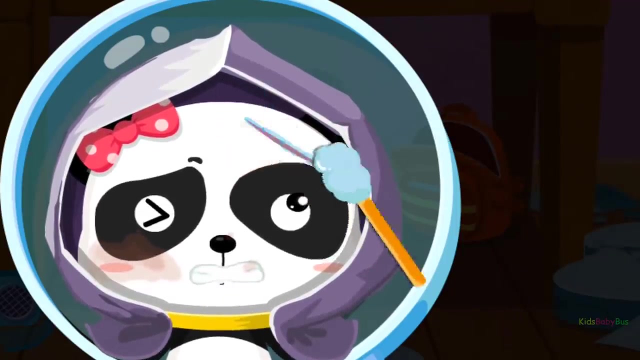 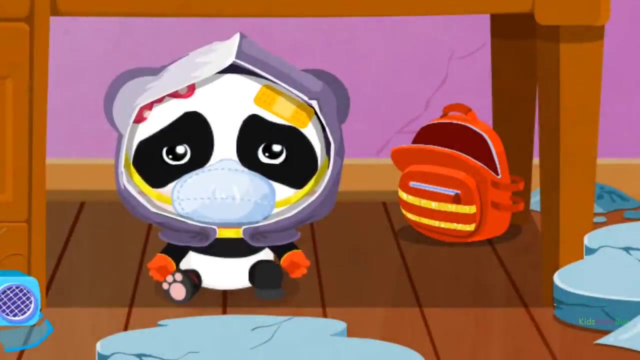 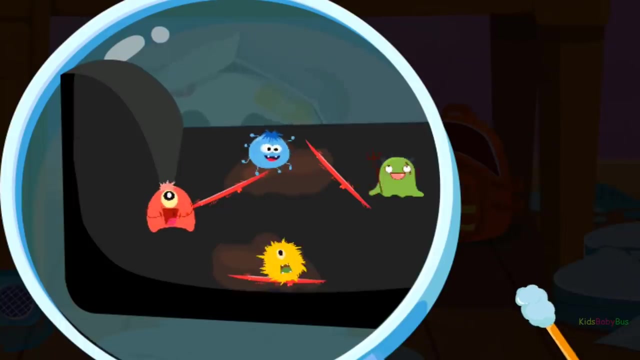 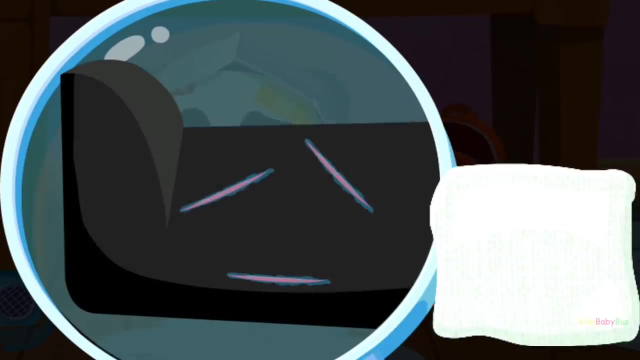 A mask can prevent dust from entering the lungs. Wearing a helmet can keep my head protected. I'm hurt. What should I do? Use the first aid kit to treat a wound. If doubt, please contact me on correspondence. I don't know. 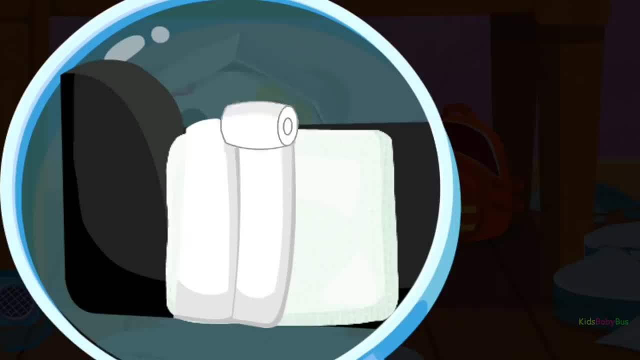 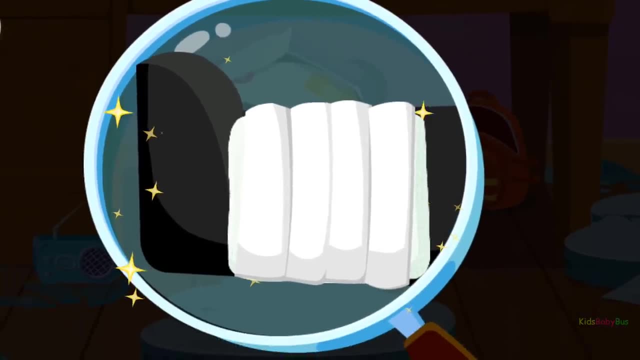 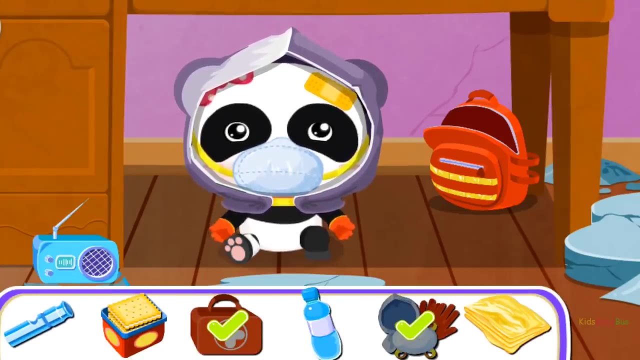 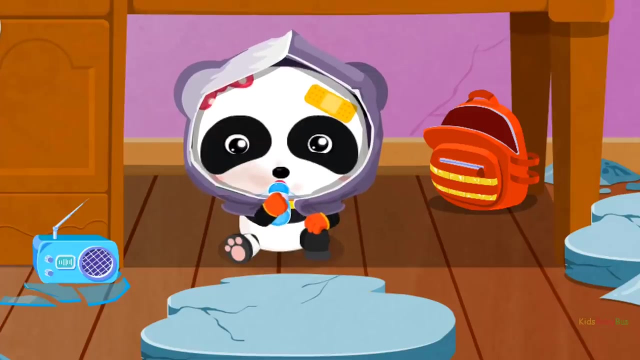 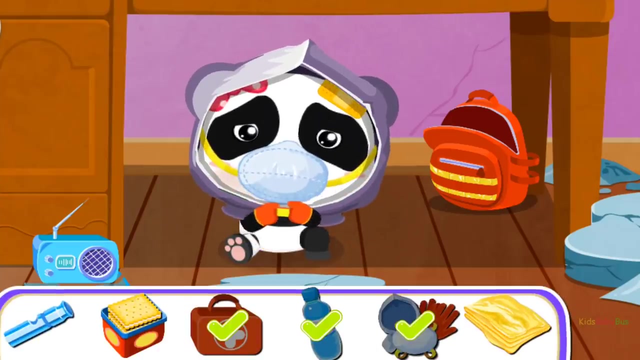 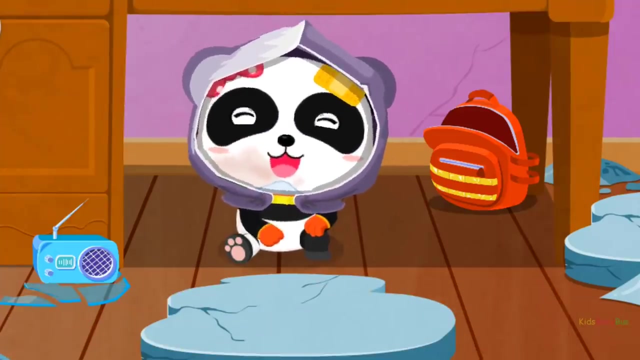 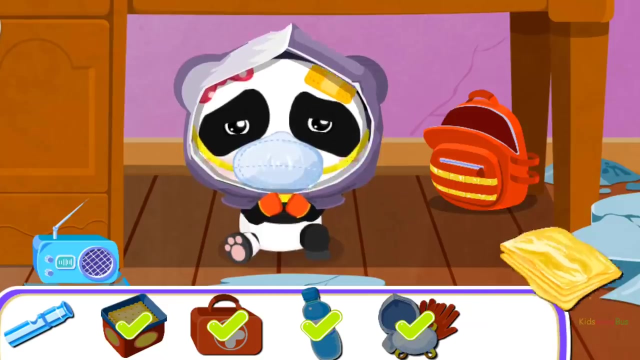 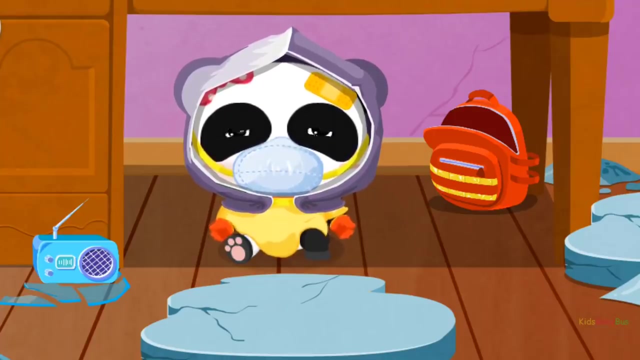 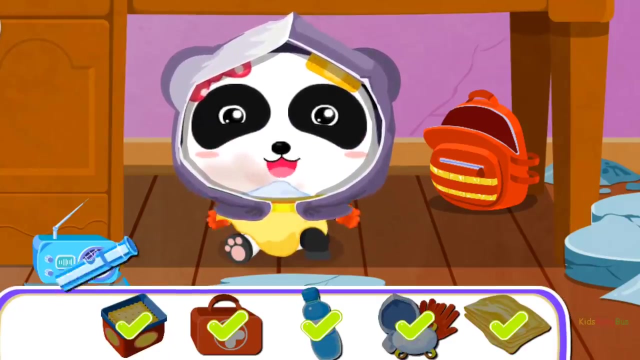 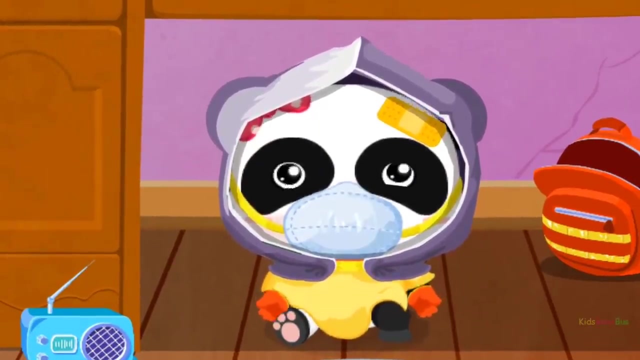 I don't know. I'm hungry. Food gives me strength. I'm cold. A blanket can keep me warm. Anyone in here- I hear someone Time to use my whistle to let them know I'm here, Don't be scared. 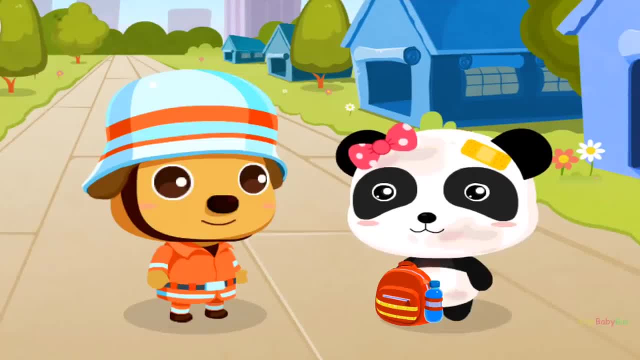 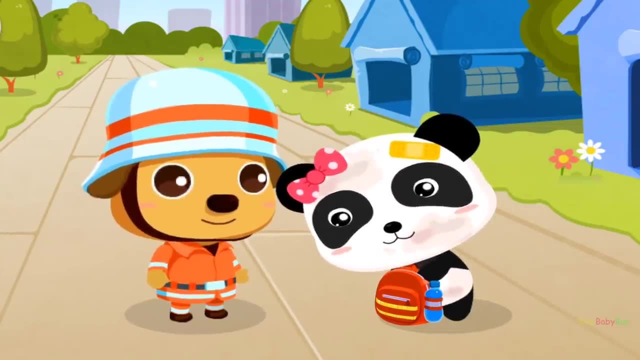 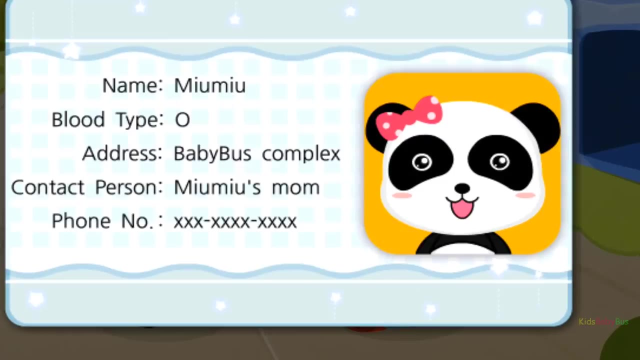 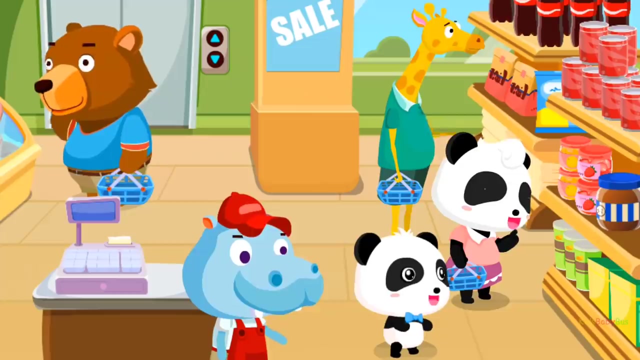 I will get you out. Do you have an emergency contact card? I can contact your parents. Yes, thank you. Carrying an emergency contact card can help you find your parents soon. Yes, Yes, The supermarket has everything. Mom, what's happening? 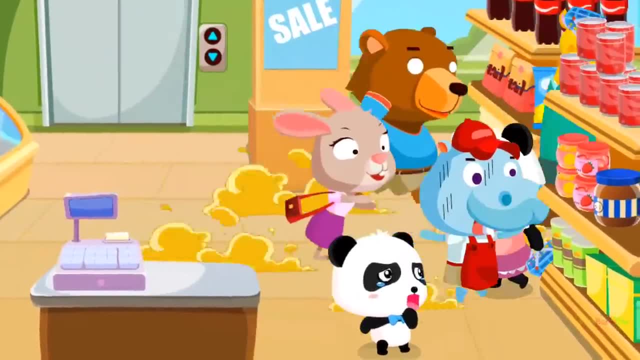 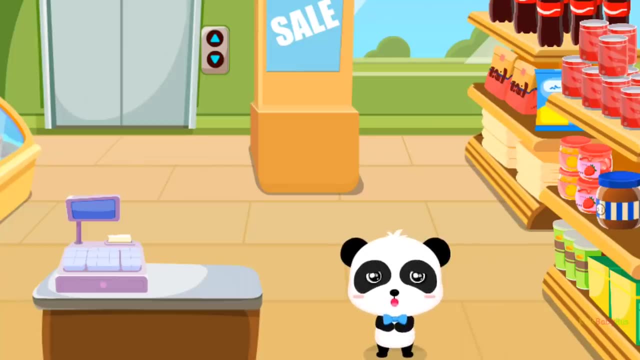 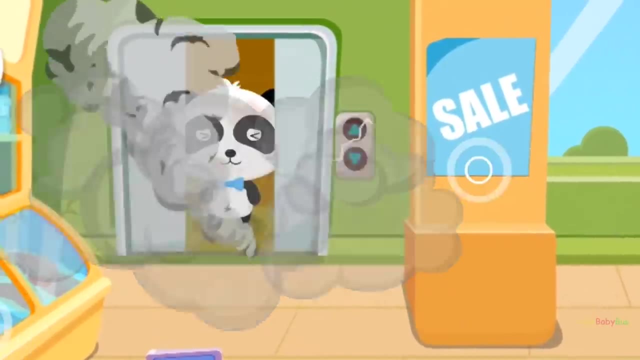 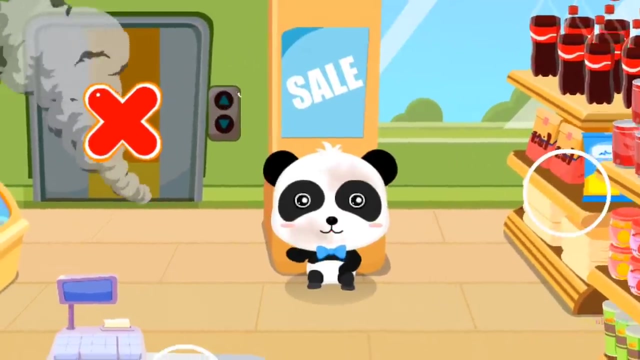 It's an earthquake, Hide, Hey Mom. where are you? What do I do now? Could you help me find a hiding place? The elevator may fall during an earthquake. Don't hide in there Anywhere else. Staying by the column is a relatively safe choice in a supermarket. 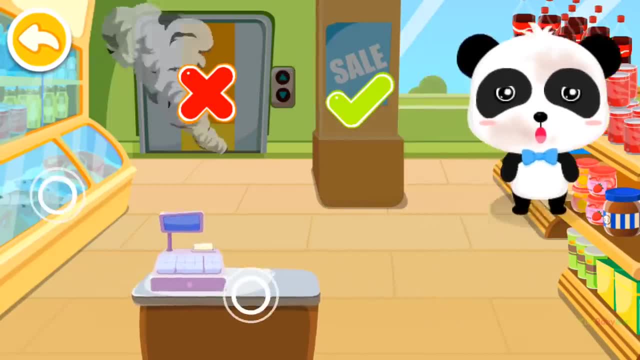 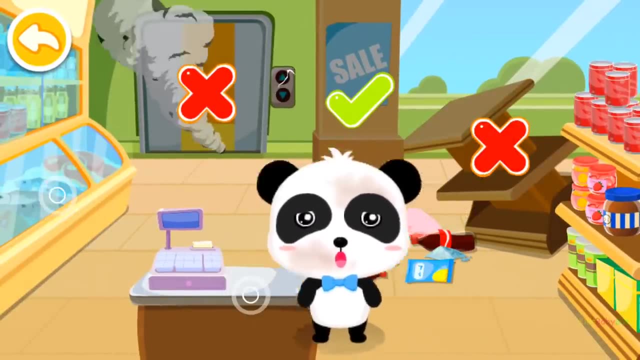 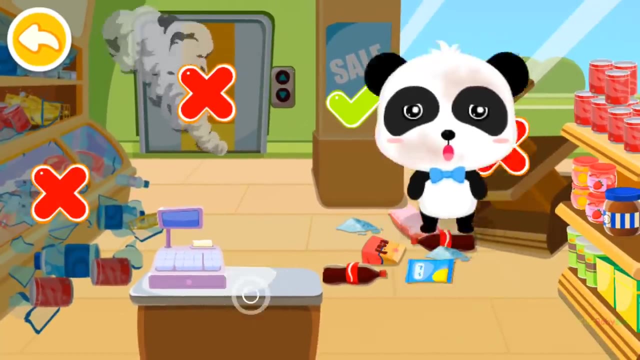 Anywhere else. Shells can fall and hit you. Please stay away Anywhere else. Stay away from the coolers with glass doors. It might break and cut you Anywhere else. Hiding by the cash register is also safe. 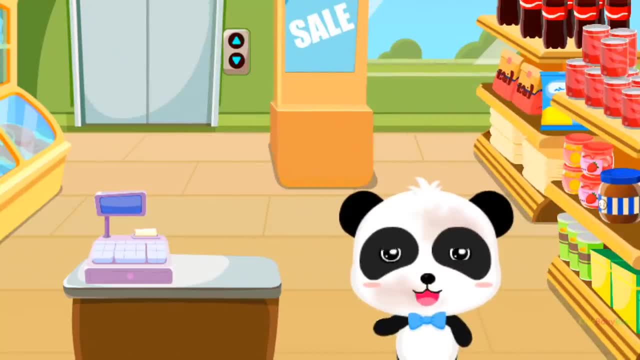 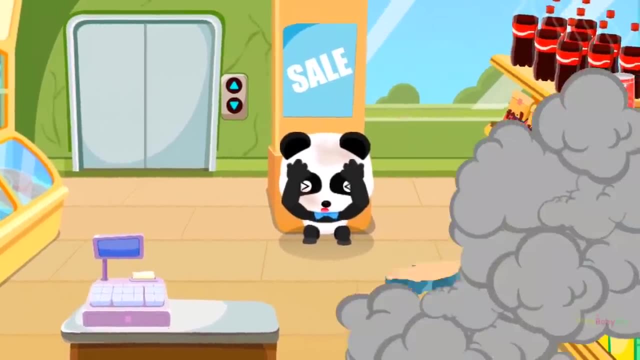 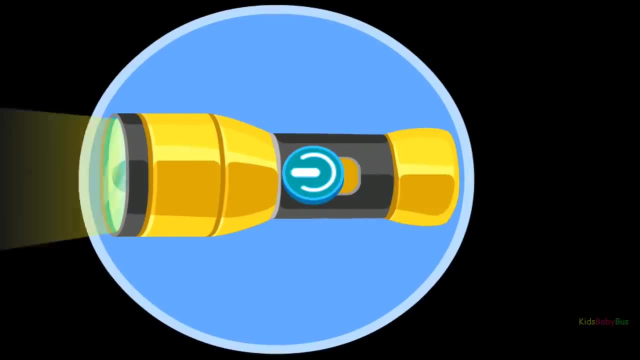 Staying by the cash register is also safe. You are correct. During an earthquake, we can hide by the post and the cash register. Let's go hide. Oh no, the power is out. Here is a flashlight. What else can I use? 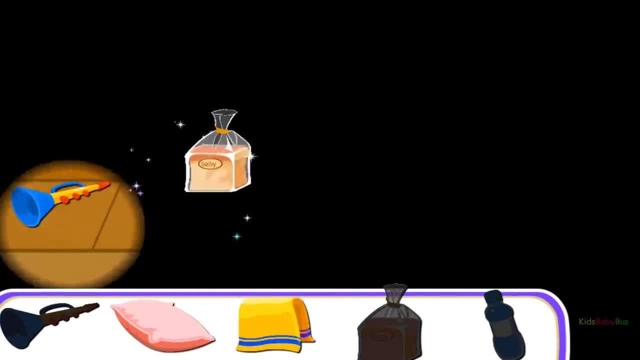 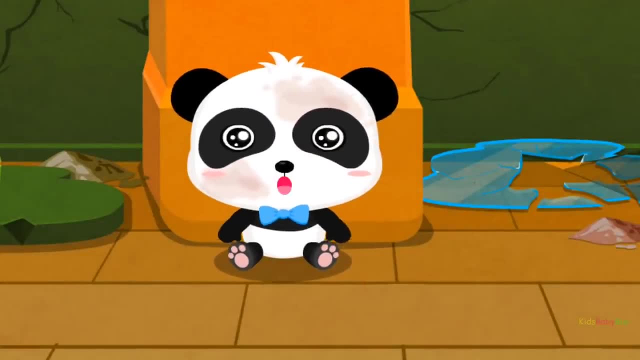 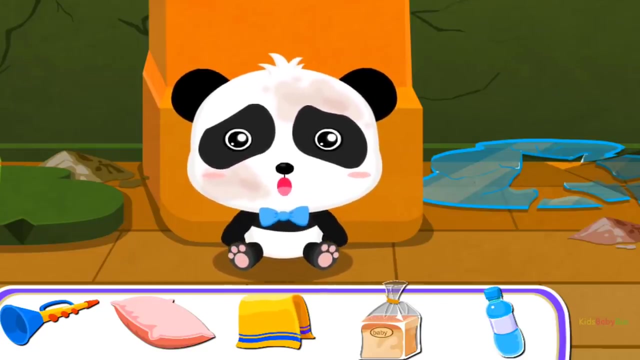 Pillow, Towel, Bread, Horn, Water. A flashlight can help me. It can help me see my surroundings While I'm waiting for the rescue crew. what can I use to protect my head While I'm waiting for A pillow can protect my head. 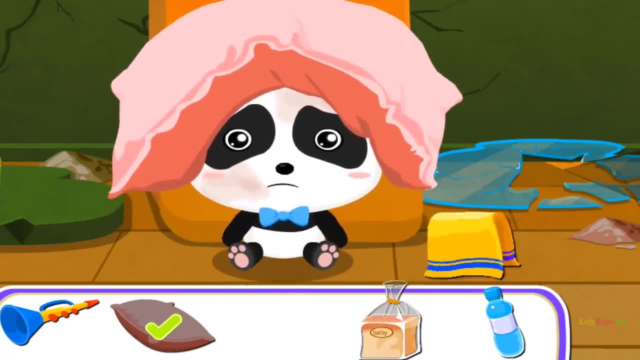 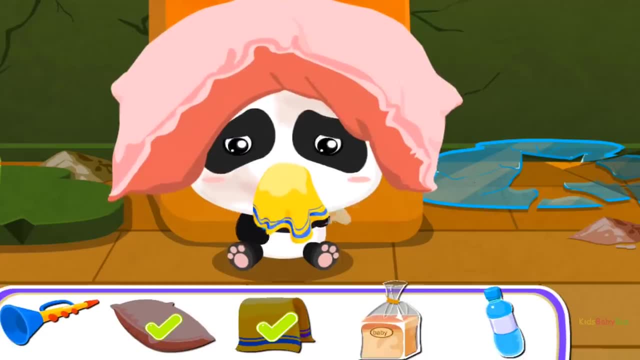 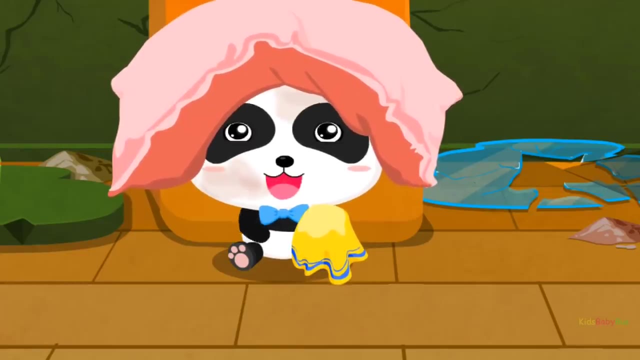 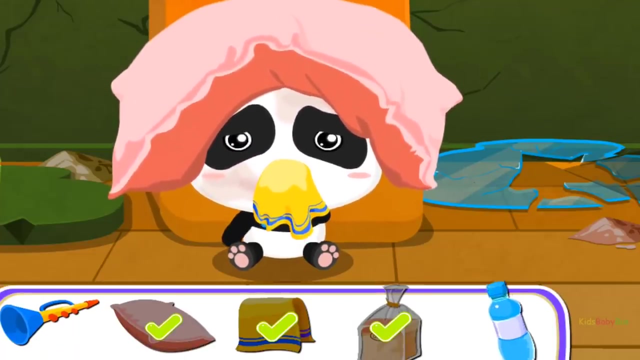 Next, I need something to cover my nose. A towel can prevent dust from entering the lungs. I'm hungry. Come and get me out. Great, I'm better now. I am thirsty, Itropic, The Ek Lazare, Drink some water and you will be better ready. 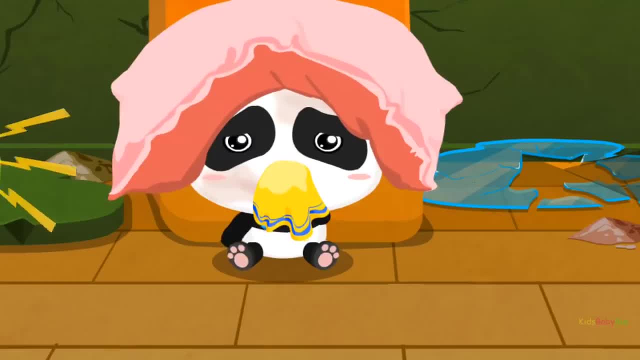 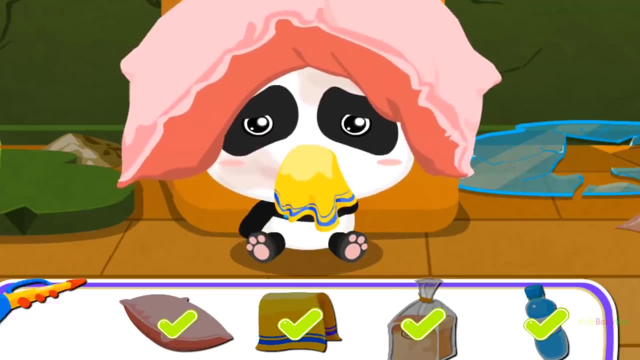 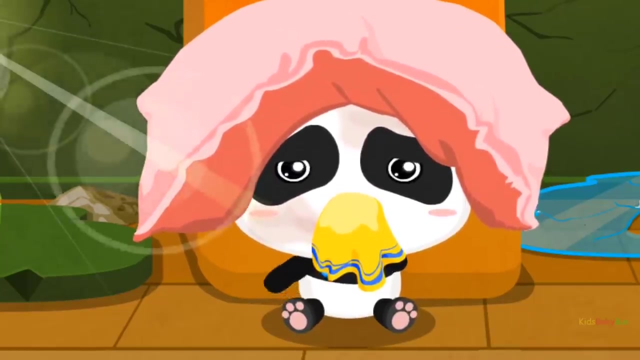 Water can keep me hydrated. Warm water can keep you hydrated. Anyone in here? Do i hear people coming? I will use the horn to let them know I'm here. No need to rush, I found you. I will get you out. Your mom is waiting for you. 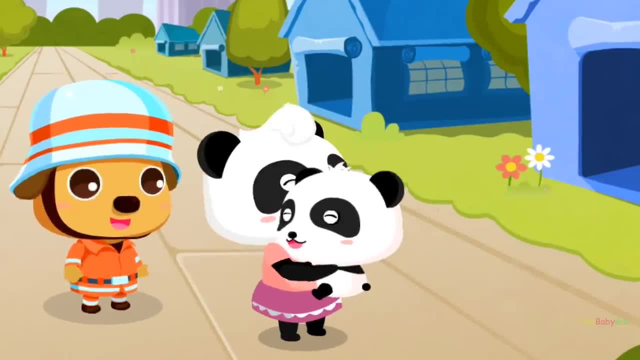 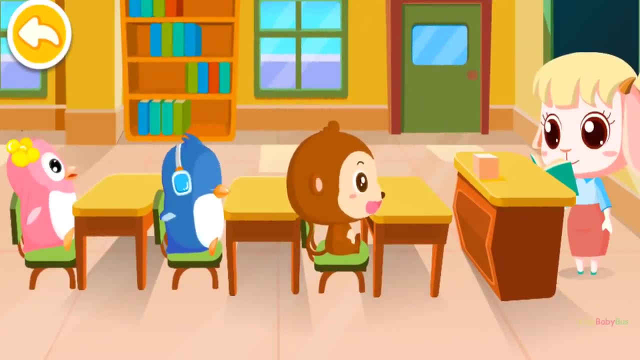 Really, Mommy Kiki, are you alright? Don't worry, I protected myself during the earthquake. Good morning children. Yes, ma'am, Is it an earthquake? What do we do now? Don't panic, I will open the door and you guys hide.